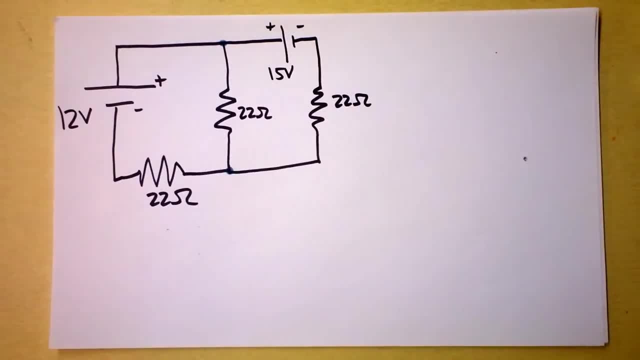 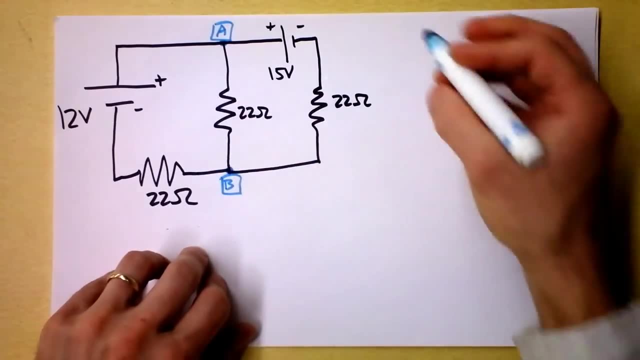 I mean, in principle, I could define any of these as junctions and they're really, really trivial. So let's define this location here as A and this location here as B, and we will say that the junctions work like this. 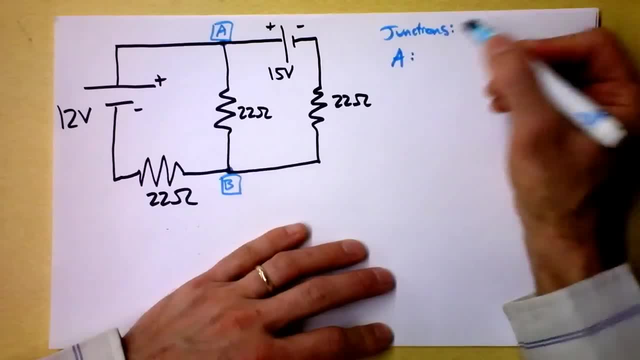 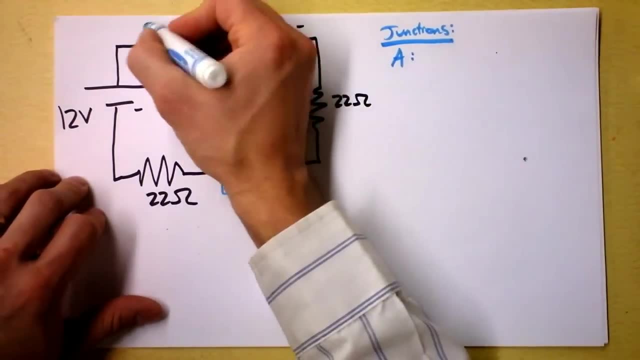 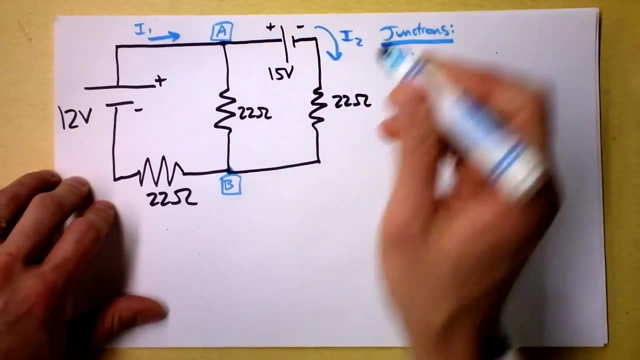 Junctions. say A gives us Junction, A gives us that. Oh, I've got to define all these currents right. So I'm going to say this is current 1 going that direction. and then I'm going to call this through here: current 2, going that direction. 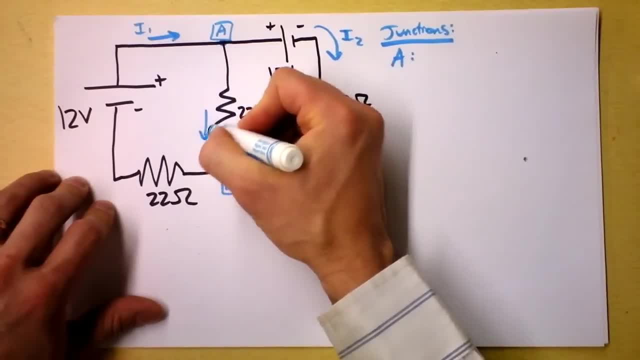 So current 2 is here as well, And then this guy. this is a separate current, so I'm going to call that current 3.. This current over here- what's this guy going through here? That current is I1 again. 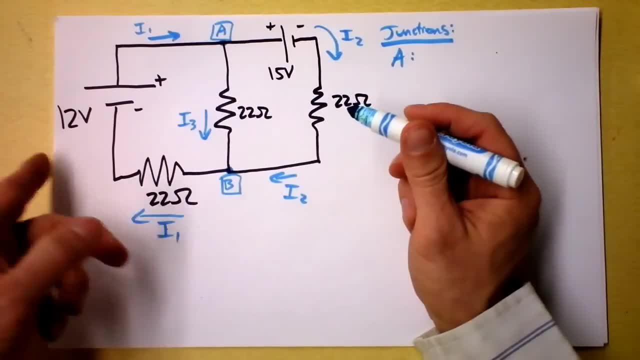 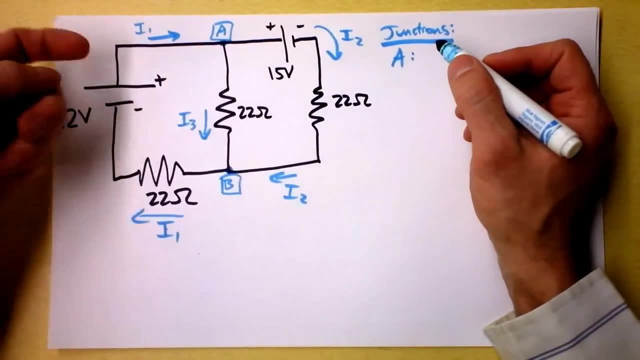 Alright. so we've got current 2,, current 3, and current 1 over in this leg, And they could, of course, be very different from one another. So junction A has current 1 going in and current 2 and 3 going out. 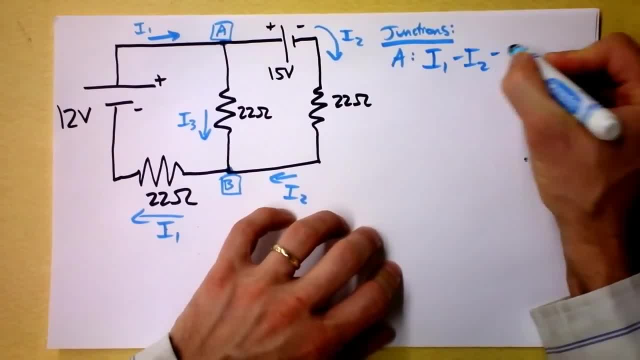 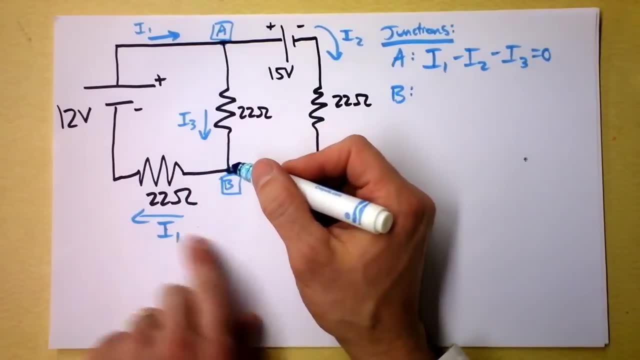 So I write: current 1 minus current 2 minus current 3 equals 0.. And then at junction B I notice that current 1 and 2 are going in, but current- Sorry, current 2 and 3 are going in and current 1 is coming out. 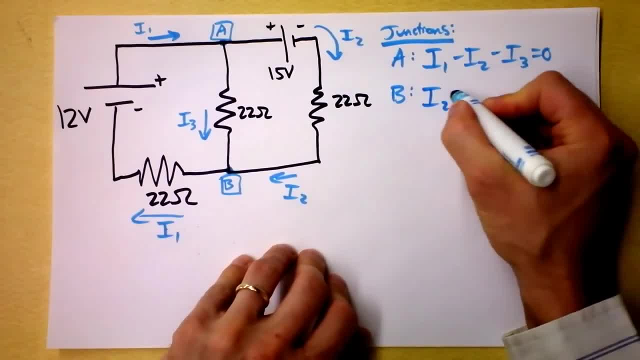 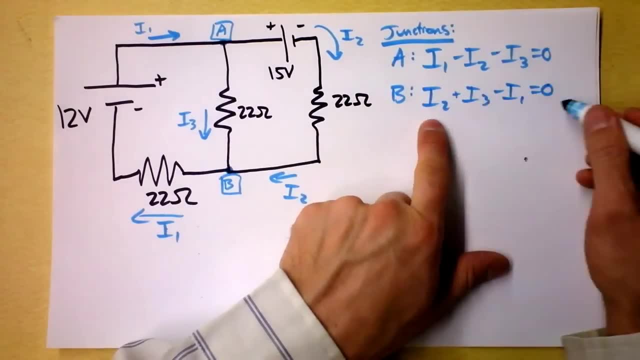 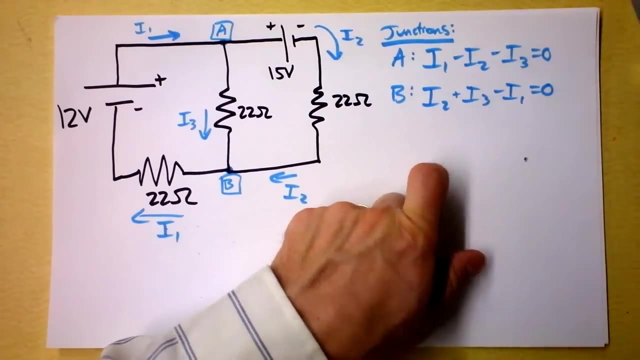 So I say, well, I say I2 plus I3 minus I1 equals 0. Notice That this equation right here is that equation multiplied by negative 1.. Alright, So that's redundant and I can just sort of cross it out. 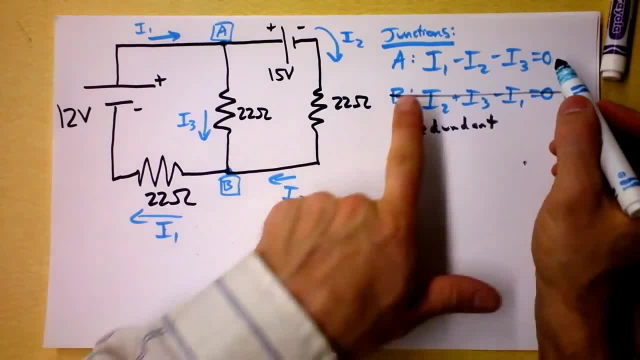 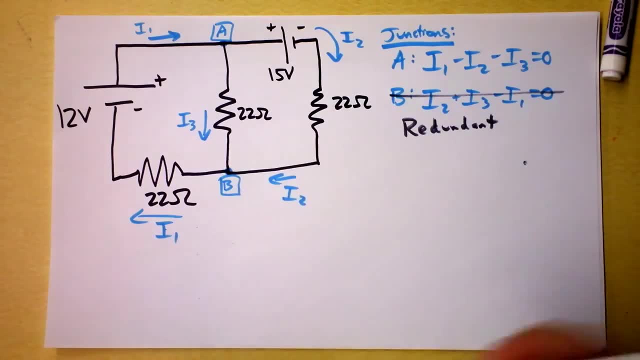 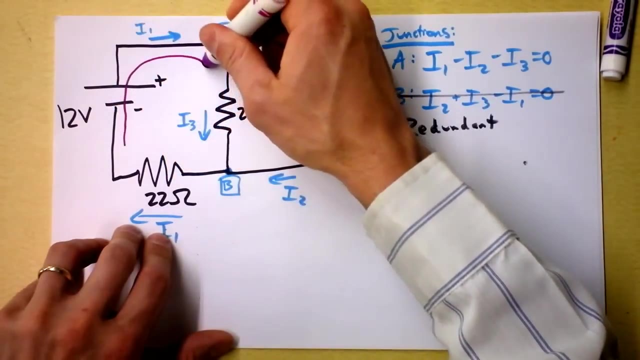 It is completely captured by the first junction. Now I have to define some loops, And I promised primrose, and here it is. My first loop is going to be here. I have to define the direction of my loop. So my loop goes this direction and I'll call that loop 1, and I'll circle it. 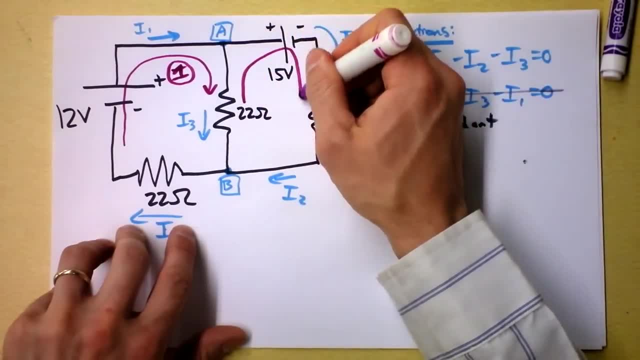 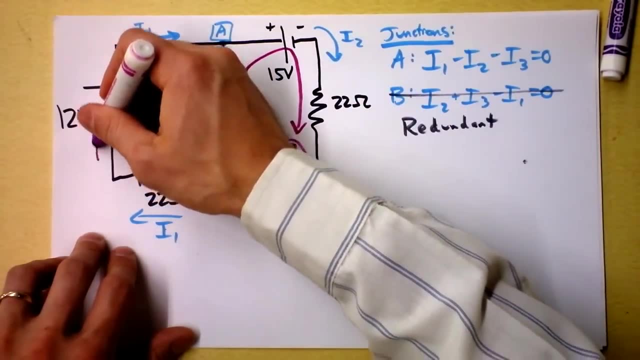 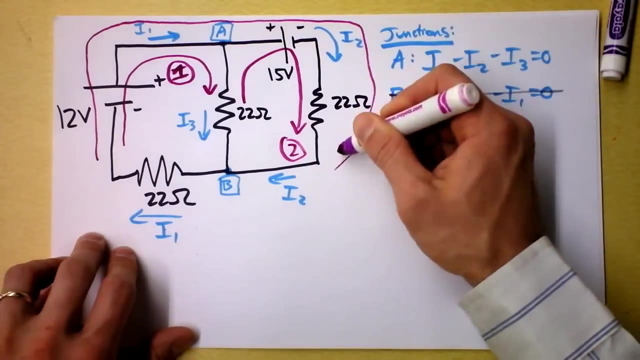 And my second loop is planning to be in here. This guy is what I'm going to name loop 2.. And then you know where my third loop is going to be. My third loop is planning on being around the entire outside. That is my loop 3.. 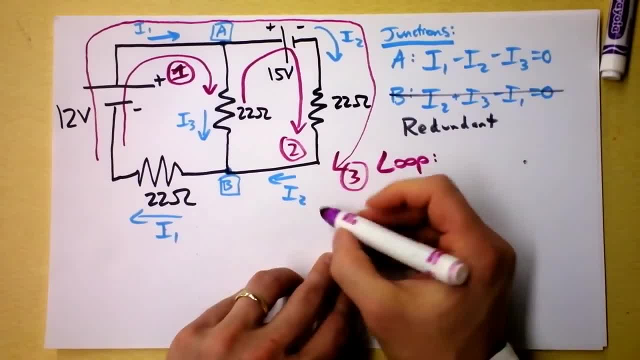 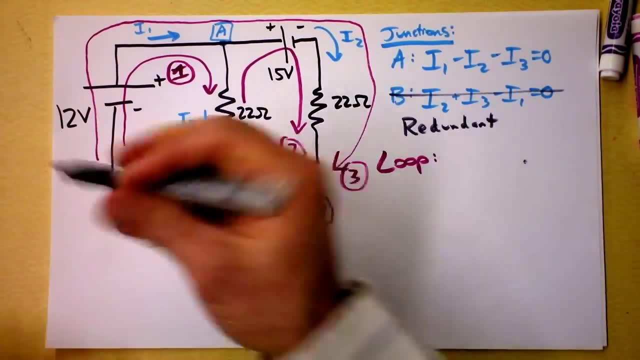 So here are my loop equations. Loop 1 says: I'm going through, I'm going to start from here Again. I like to just define something to be 0 volts. I'll just call that 0 volts. And the loop equation says: if I go around a loop and I get back to 0 volts, 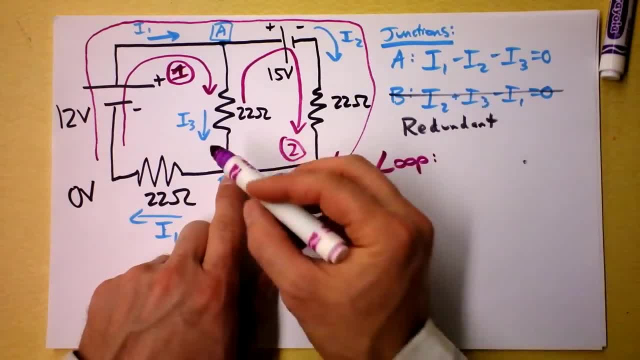 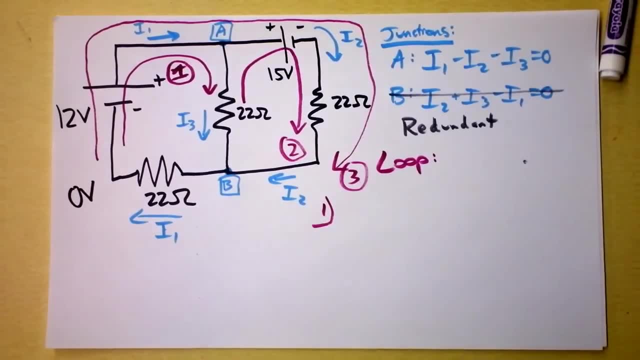 I've got to get back to 0 volts, Or if I'm starting from over here, like I have to start at junction B for loop 2, I'm going to get back to whatever that voltage is. but I'm going to get back to that value by gum because energy is conserved. 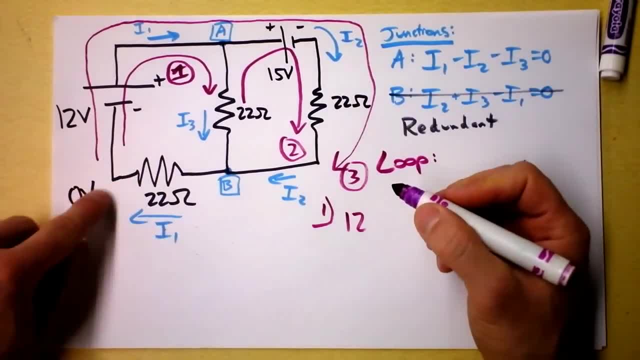 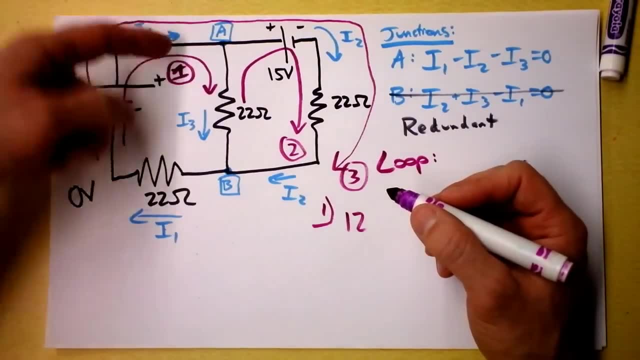 So for loop 1, I find that I get 12 volts addition because I'm going through that battery, that direction, And then, as I continue in this loop, I've got an equipotential here, as I've got a conductor. 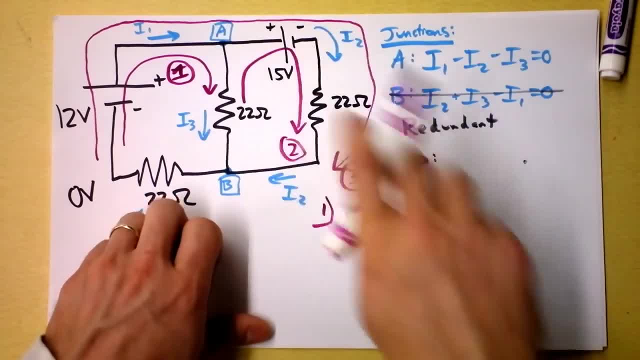 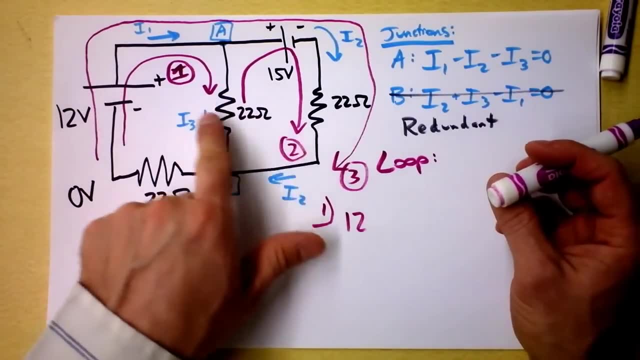 and then I drop my voltage because I'm going through a resistor in the proper direction- Notice that current 3 is pointing that direction- And I'm dropping my voltage, assuming that I've defined these currents correctly. But guess what? I didn't. 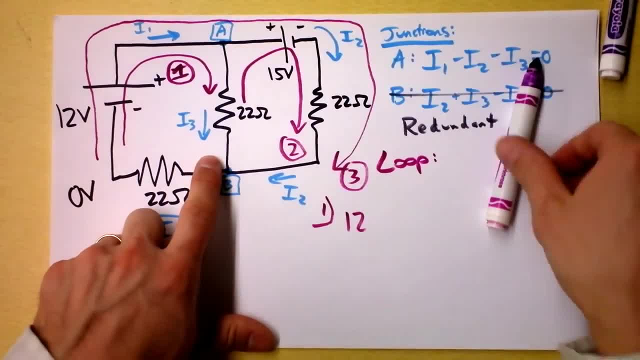 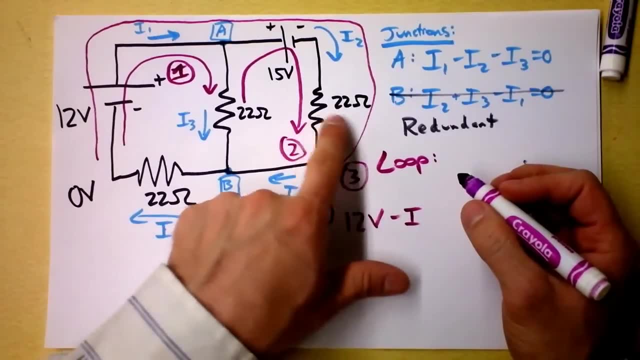 So that's going to be a fun surprise. But assuming I'm going that direction, my voltage will drop. So I have to subtract the voltage drop on this resistor, Which is- Oh, I'm just going to call them R because they're all the same. 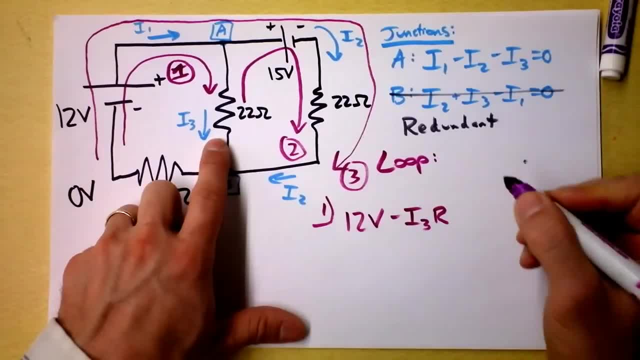 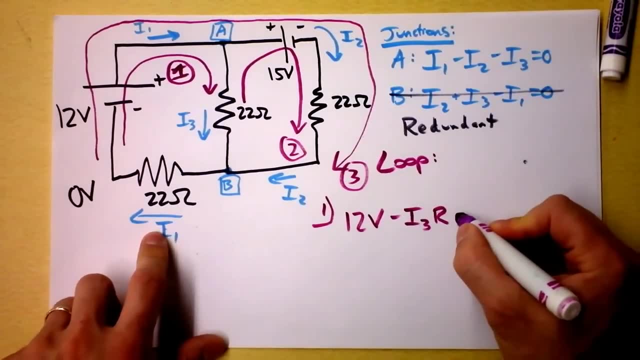 We can plug in for that later. It's going to be I3 times Ara. And then, as I continue this direction, I'm going through this resistor in the direction of the current, So I'm dropping my voltage again And that's going to be I1 times Ara. 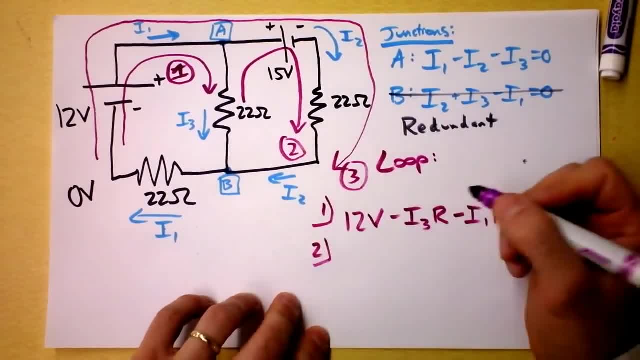 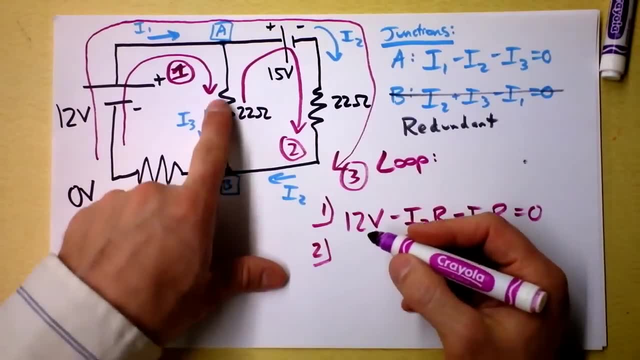 All that stuff has to equal 0 in loop 2.. I start from this point and I say I'm going through that resistor opposite the direction of the current, So I actually get a voltage increase. According to my statement, I'm going to have to get I3 times Ara. 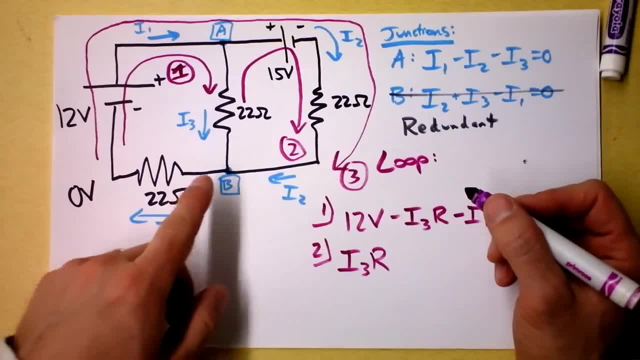 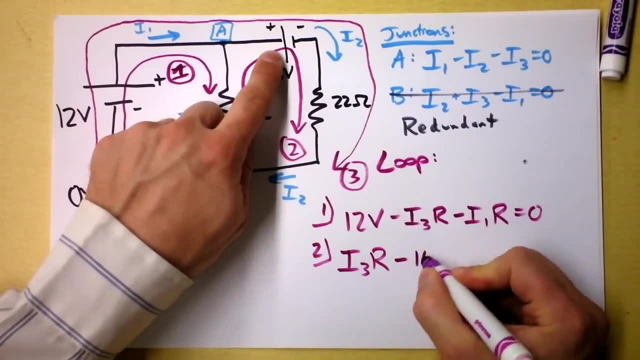 And it's positive, because I'm going the wrong way through the resistor, So it's not a voltage drop, It's a voltage rise Here. I'm also going the wrong way through that battery, So I'm going to subtract 15 volts. 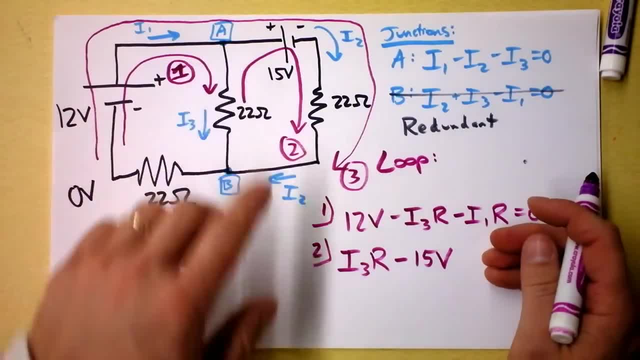 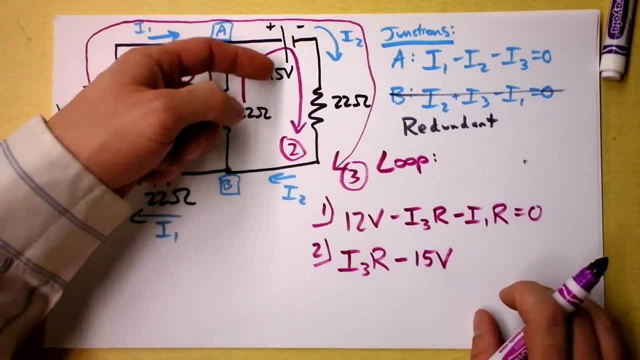 Weird, Weird. Okay, so maybe I made some of these definitions wrong. But that's okay, I'm just going to get minus signs in my variables. I'll still be able to tell you what the current is and which way it's going. 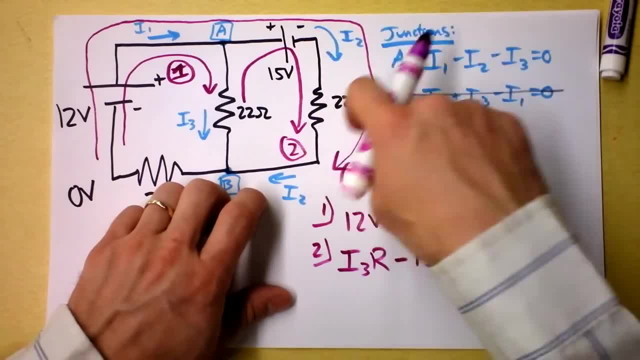 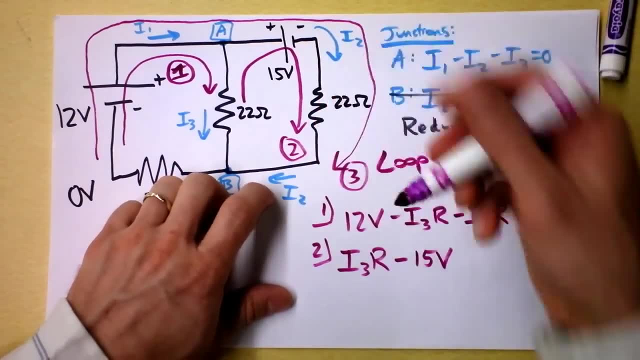 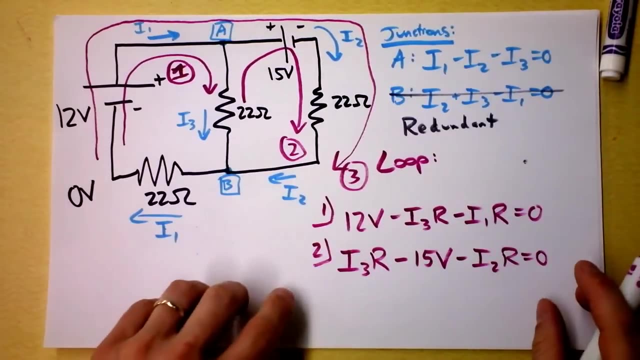 So then, as I continue through this resistor- thankfully I'm finally going the proper direction- I'm going to have a voltage drop right here through that resistor, So that's going to be minus I2 times Ara equals 0.. And then I'm going to get loop 3 going right here. 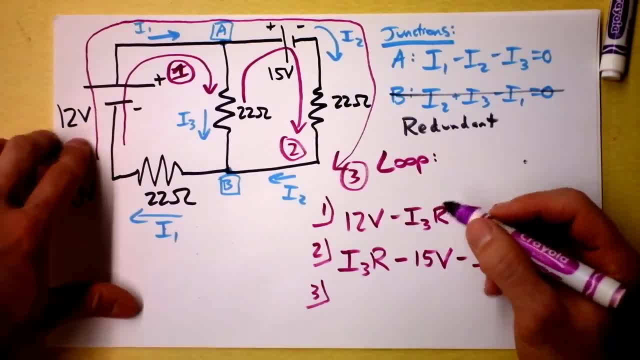 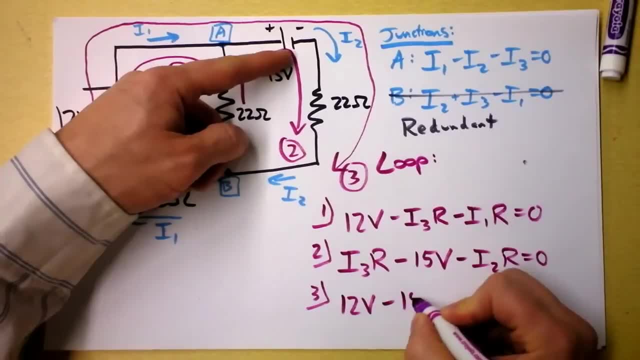 Loop 3 starts here and goes all the way around the outside of the circuit. I get 12 volts And then I'm going through this battery the wrong direction, So I subtract 15 volts And then I'm going through this resistor as a voltage drop in the direction of the current. 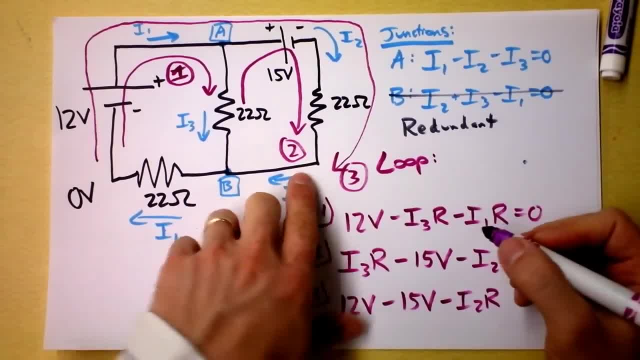 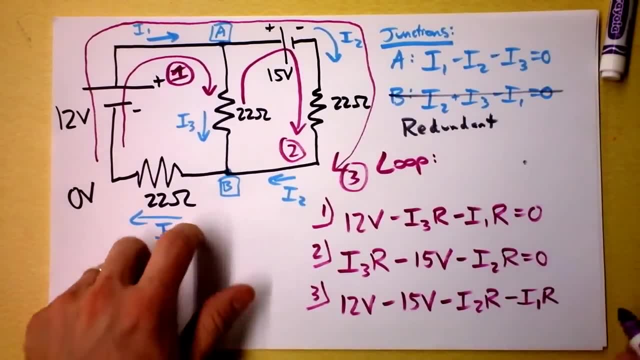 So I subtract I2 times Ara And my final resistor- I need to go through- is going to subtract I1 times Ara. I'd like you to notice something: This is equal to 0.. I'm going to draw a line right here. 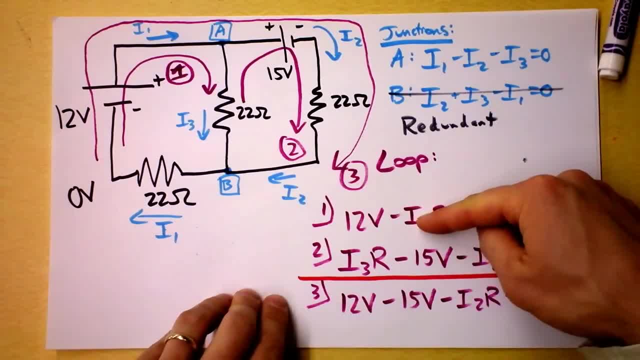 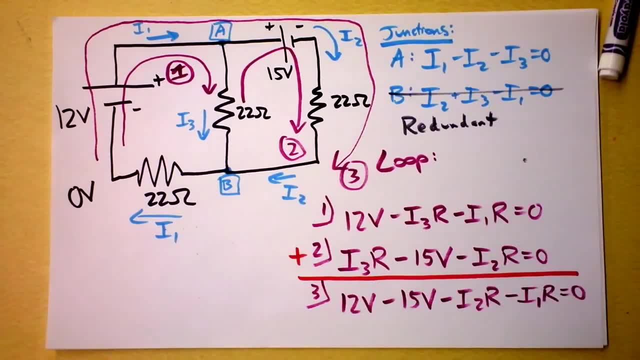 And I want to point out what's going on. If you take this equation and add this equation, you actually get this equation right here. So again, we have a redundant equation, This one plus this one- Check it out- We got a 12 volts. 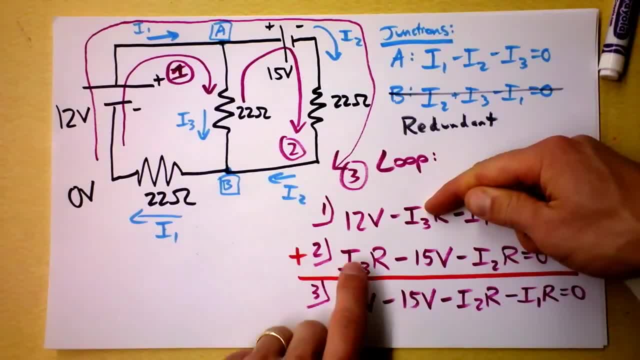 We got a negative 15 volts. We got an I3R minus and an I3R plus, So those guys don't appear. And then I'm subtracting: I1R Boom right there And I2R right there. 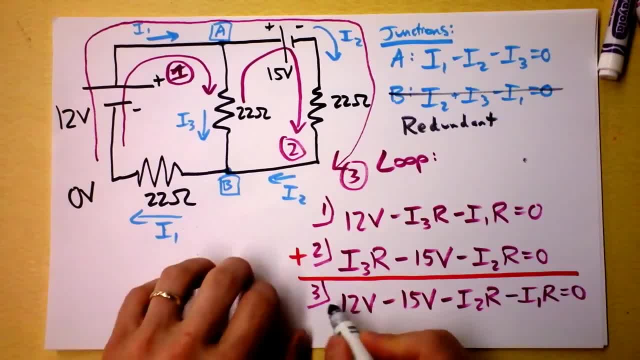 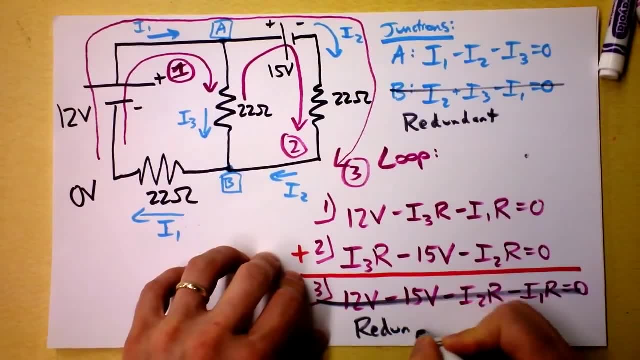 So this again is a redundant equation, And you find this a lot with Kirchhoff's rules. They are beautiful, But you have to be careful, because sometimes you get too much information And it is simply a waste of your time. 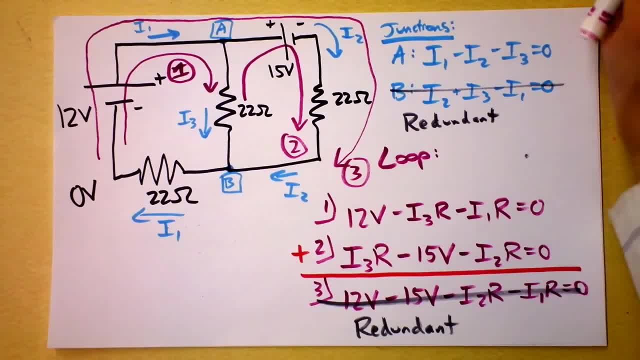 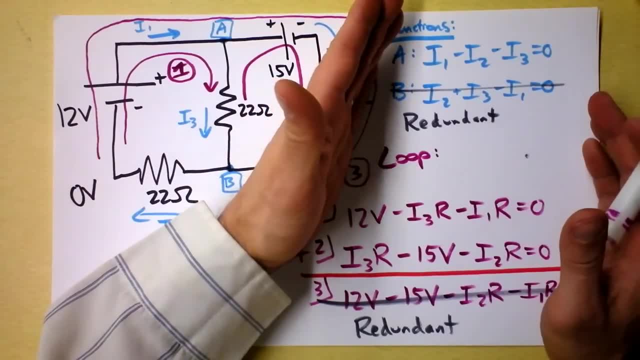 As you get more and more, More experience with them, you'll find that they can be really efficient if you know where to look for these redundancies. So I'm going to take these equations And I'm going to do a bunch of equation analysis. that's not really physics. 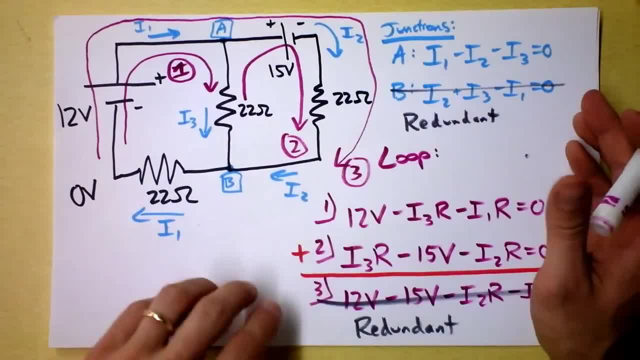 It's simply math, And I'm going to do it in a kind of clunky, straightforward way, Nothing elegant, And then we'll come back. We'll be able to say what all these currents are. I'm not going to solve for them. 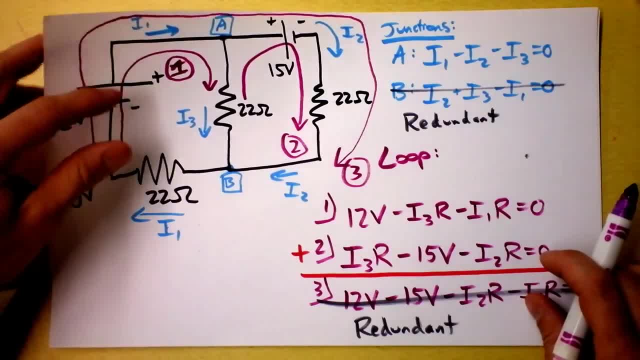 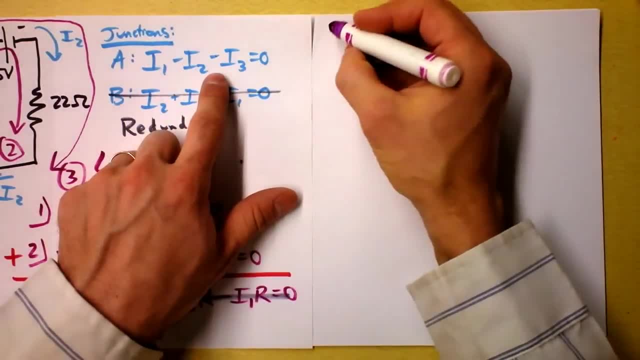 But we'll find that some of them are negative in a really explicit way. So let's take these equations. We have only three equations And my intention is to solve this one For I3. And I'll Well, maybe you'll see why. 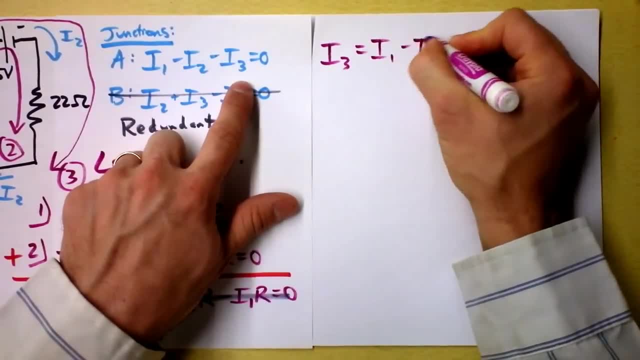 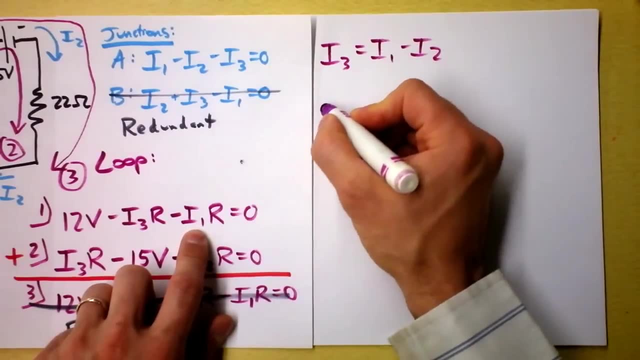 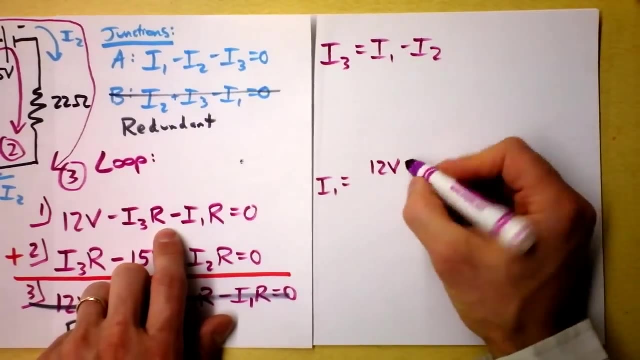 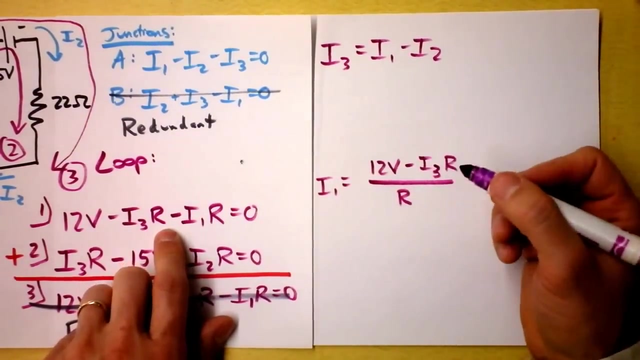 Anyway, This is I3.. It's got to be I1 minus I2. And my next plan is to get this guy solved for I1.. So that says that I1 equals. Well, it's going to be 12 volts minus I3 times Ara divided by Ara. 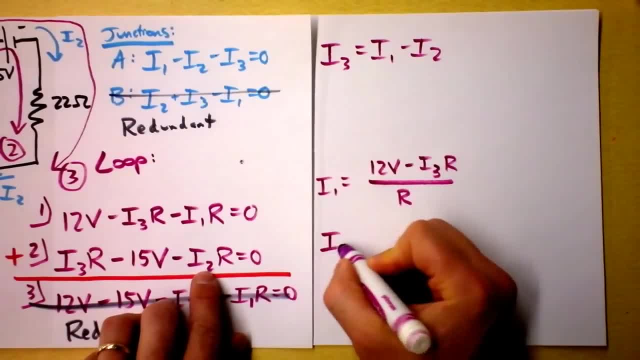 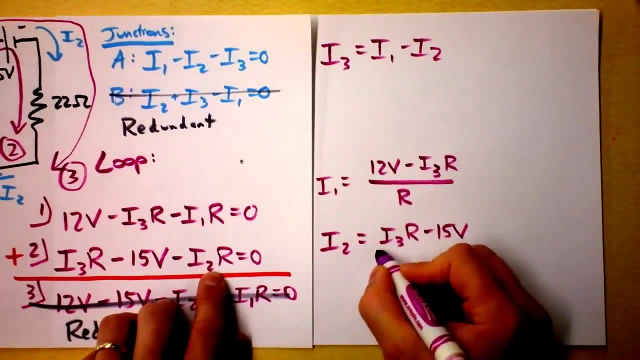 Right, Okay, And then if I solve that, If I solve this guy for I2, I2 will be I3 times Ara minus 15 volts, the whole thing divided by Ara. Naturally, we did this so that we could plug into the above equation. 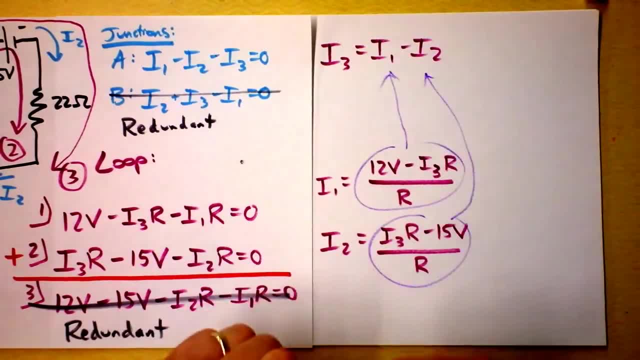 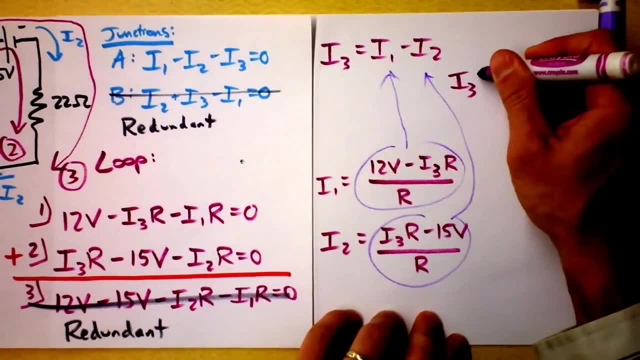 Take these guys into there And you'll see that we actually have an I3 that we can solve on its own. We find I3 equals Oh man. Well, the whole thing is divided by Ara. So that's nice. 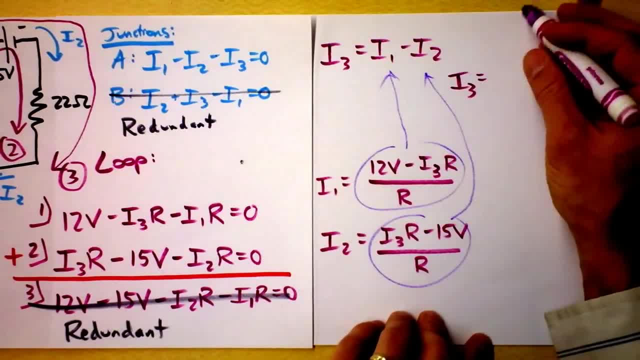 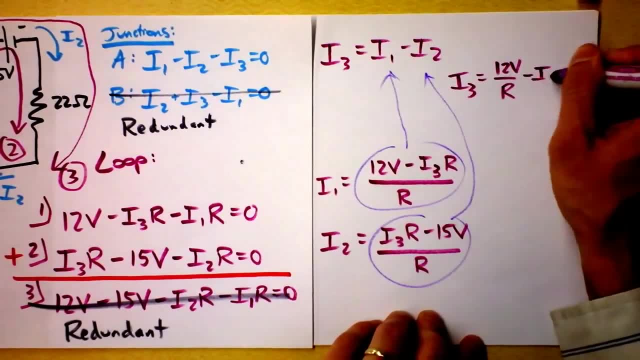 I'm going to write it like this. How should I write it? Nah, I'll just write it like this: I got 12 volts divided by Ara minus I3. And then I have to continue going this way, except I'm going to subtract. 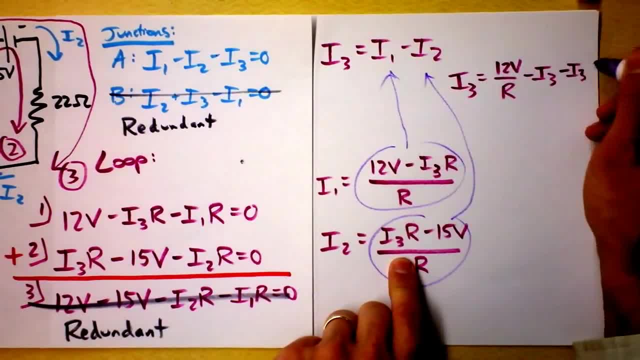 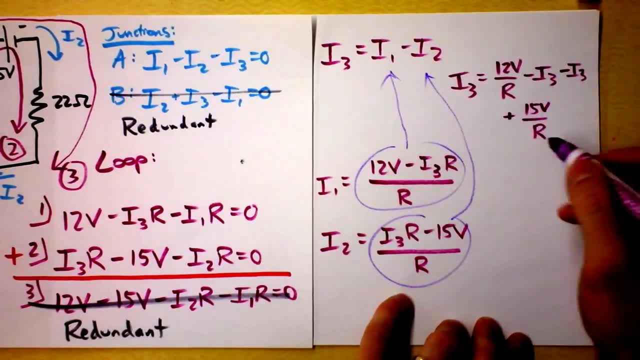 And that says minus I3.. And then I add plus 15 volts divided by Ara. Now if you look at all, If you look at all this mess right here, it looks like I've got two I3s over there. 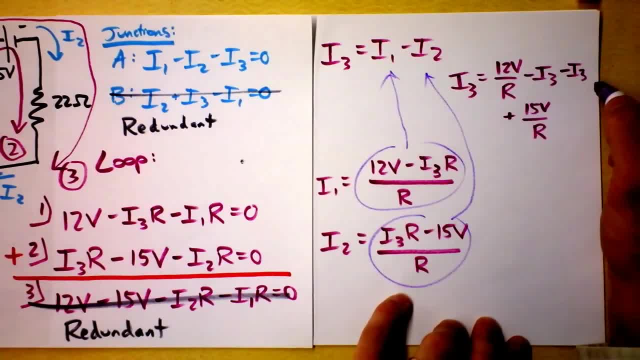 So I could make. What am I going to do? I'm going to add two I3s to both sides. So I say that three I3 is- Oh my goodness, This is way too much detail. How many? 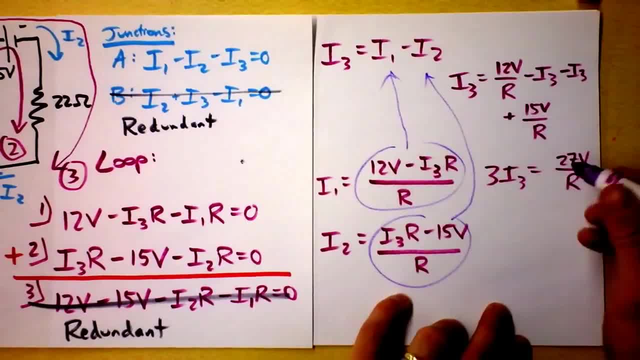 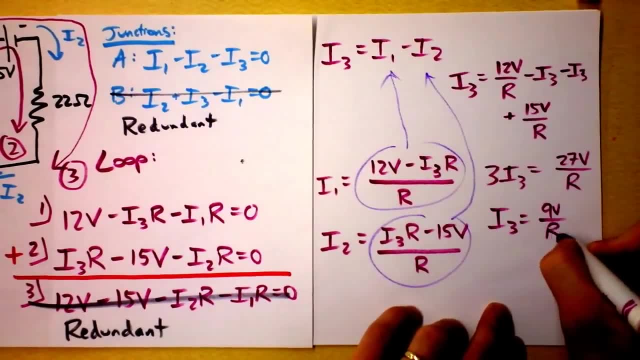 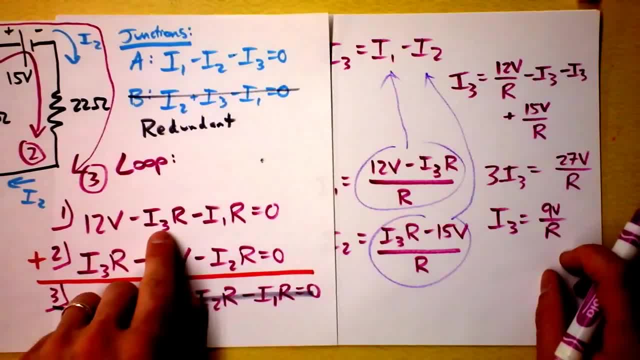 Where do you want to go? You've got your I3 now, So you can go to this equation and solve for I1. And you can go to this equation and solve for I2. Then you'll know all the currents.